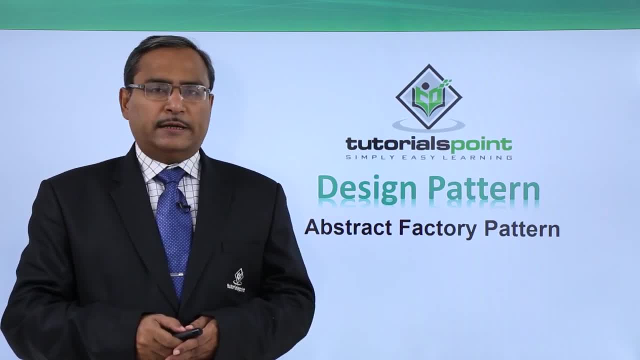 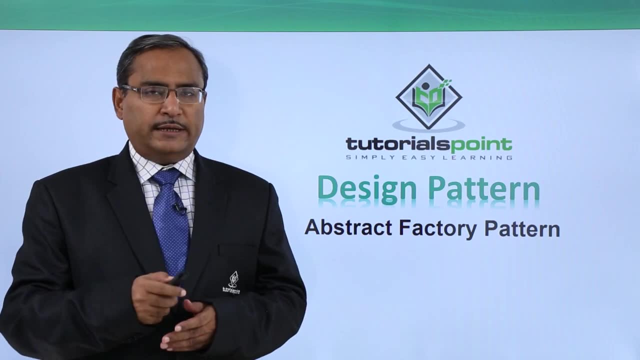 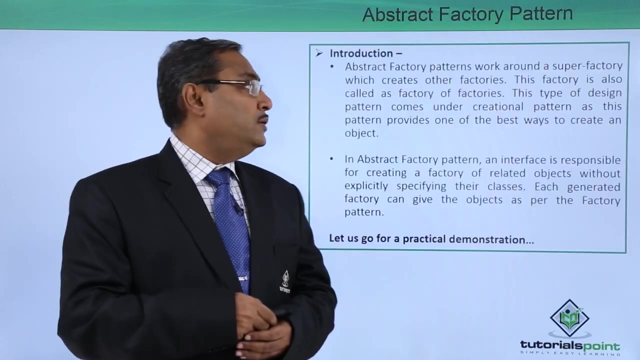 Abstract factory pattern. In this abstract factory pattern we are going to discuss and going to deal with a super factory which will create other factories and those factories can create other factory of factories. So that is the concept of abstract factory pattern. 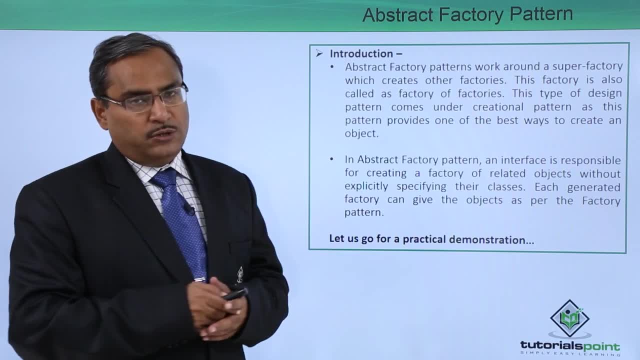 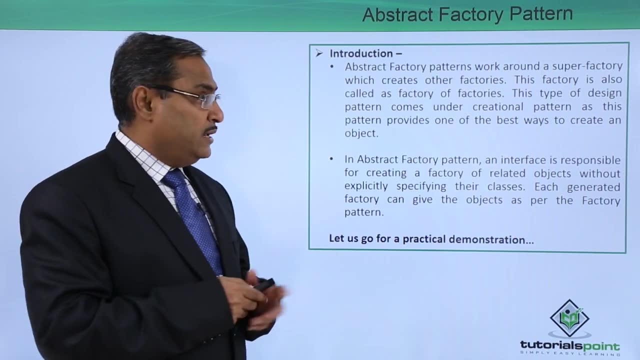 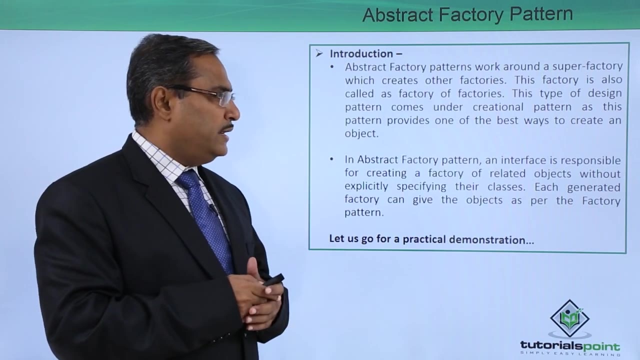 So abstract factory pattern, work around a super factory which creates other factories. This factory is also called a factory of factories. So this type of design pattern comes under the creational pattern and as the pattern provides one of the best ways to create an 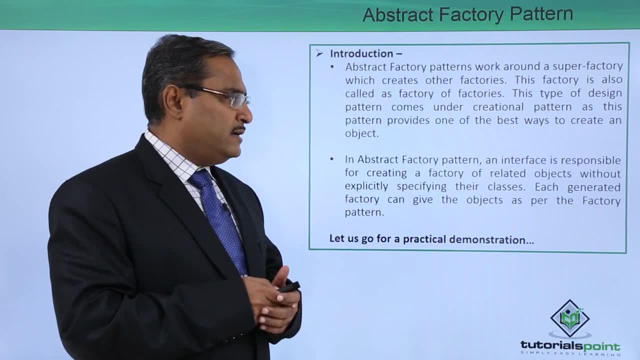 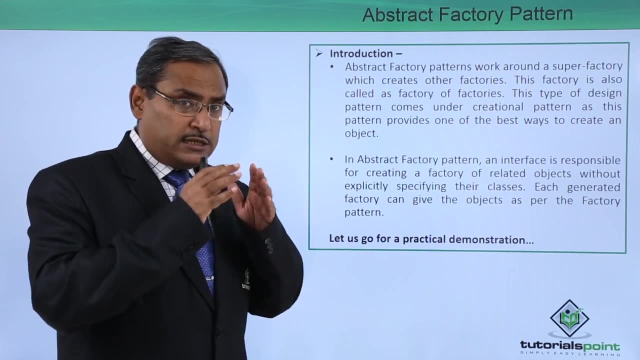 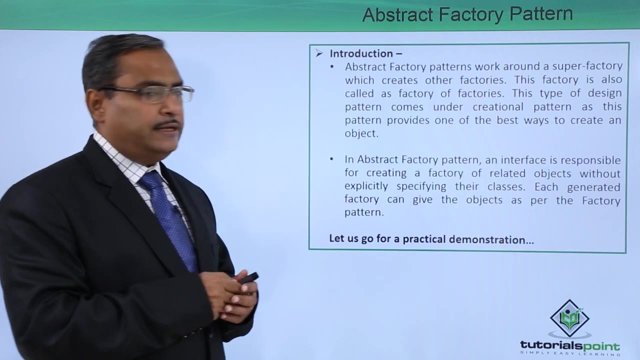 object In abstract factory pattern. an interface is responsible for creating a factory of related objects without explicitly specifying their classes, and each generated factory can give the objects as per the factory pattern. So there is a nice way to generate the super factory and then super factory will create. 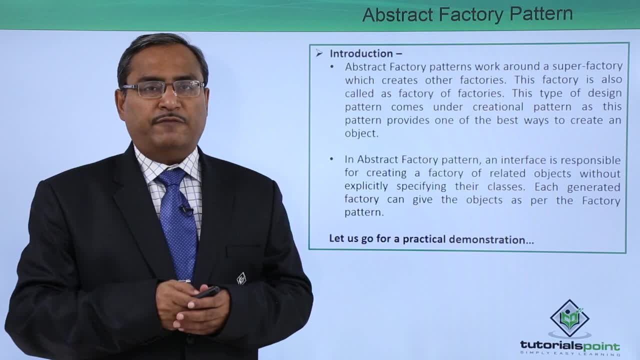 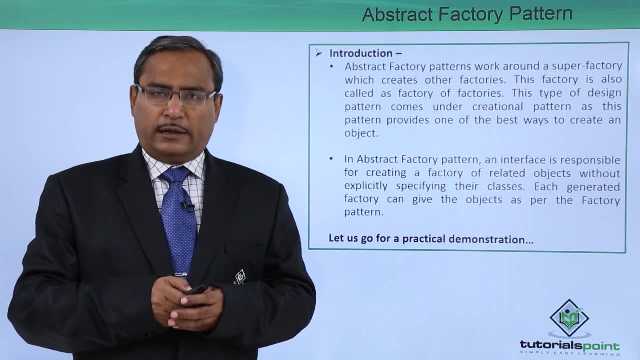 other factories, and each and every factory can create factory of factories. So that is the basic notion behind this abstract factory method. So we shall go for a demonstration, practical demonstration, to show you that in Java, how such design pattern can be implemented. 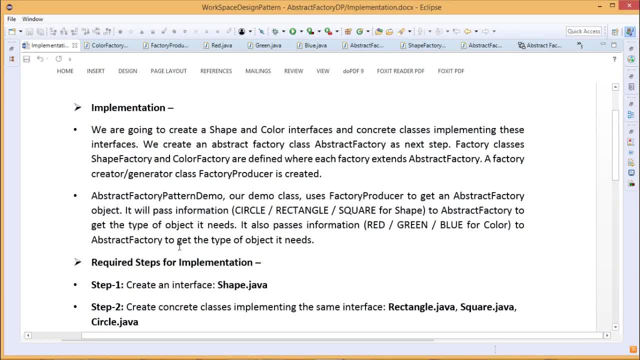 So here is the demonstration for you. In this program we shall implement abstract factory design pattern And we are going to create two interfaces: one is the shape, another one is the color and concrete classes, implementing these interfaces And we shall create an abstract factory class. 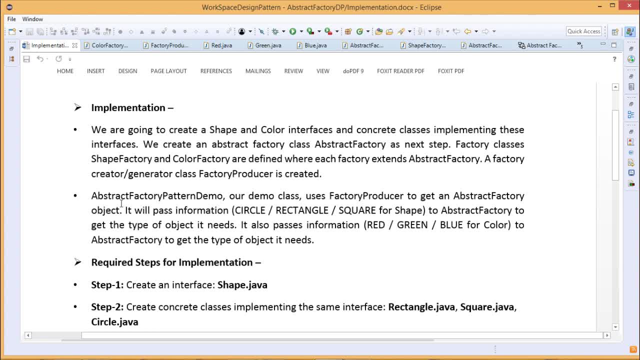 that is, the abstract factory. as the next step, And factory classes- that is, the shape factory and color factory- are defined. where each factory extends abstract factory, A factory creator or the generator class, that is, the factory producer, will be also created. An. 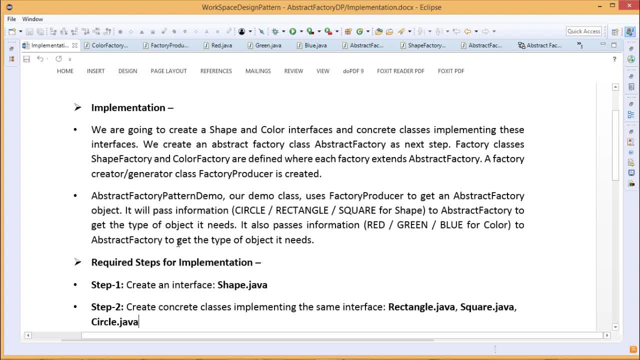 abstract factory pattern demo about. this is the next step, So we shall create an abstract factory demo Here. let us start to start, which is go ahead. all right, Your first step is to create an abstract factory, but first of all we want to create the object. 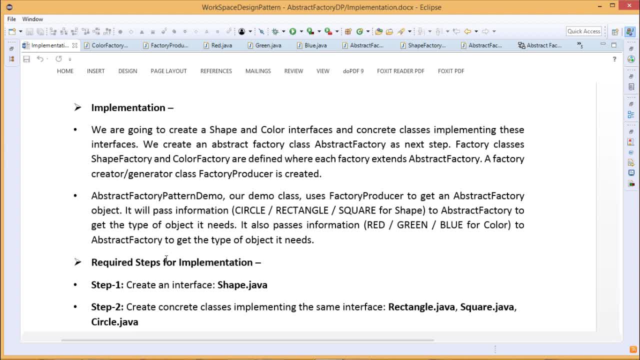 called a object. So this is, when we create an object, we only need to create the object and keep in mind that we are already creating a robotic computer. In fact, the user base usually is 3 nos in various experiences. Now, as much administrative forces apply here as 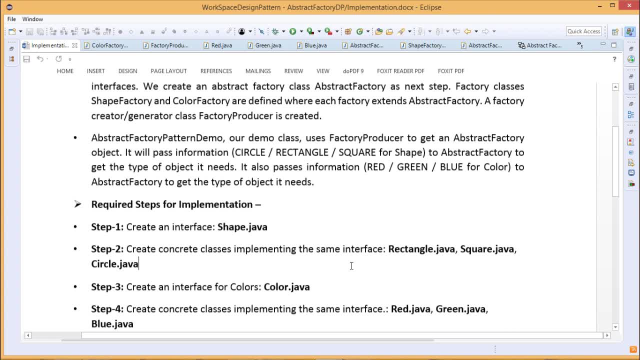 take function to some information. A component of this is made entirely random as there are four category terms. whether we count the particularuggling element and either save them or not, The pictogram of this pattern is the best to run and save in this example. 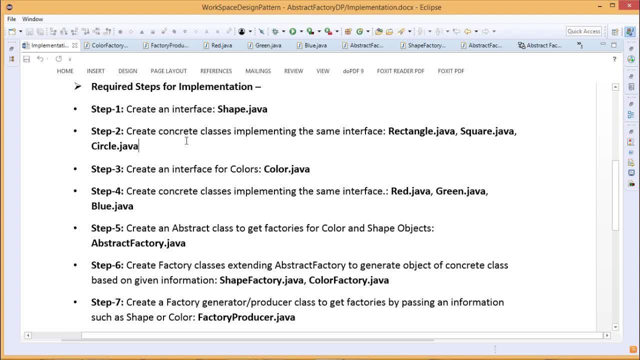 we are having certain number of states and we'll be discussing one by one. so at first we shall create one interface, that is the shapejava and its implemented implementing class that is a rectanglejava, squarejava and circlejava. so at first we are going for the shapejava. 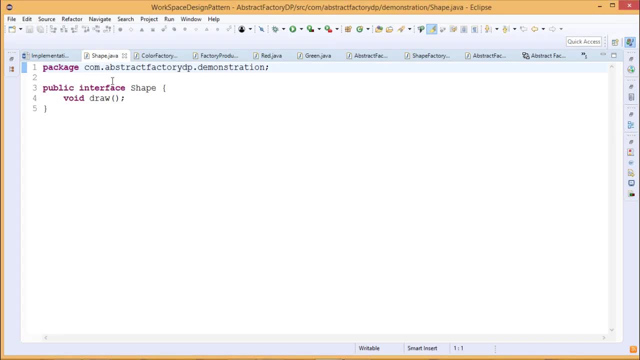 so this is our class here, shapejava, and this particular interface, this particular interface, shape, is having only one method. that is our draw. so we have discussed this shape interface here, so now we shall go for, say, circle. so circle is one of the classes implementing the shape interface. 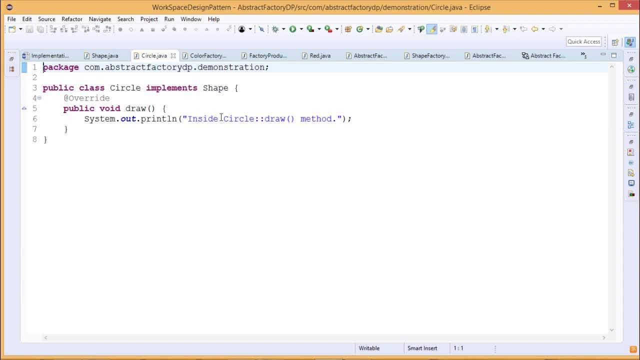 which is rewriting the body for the draw method will be another two classes, so one will be the rectangle. so in case of rectangle- so it is having this class, rectangle implements shape and there's a draw method has been rewritten here- then you shall go for another one, so that is a square. 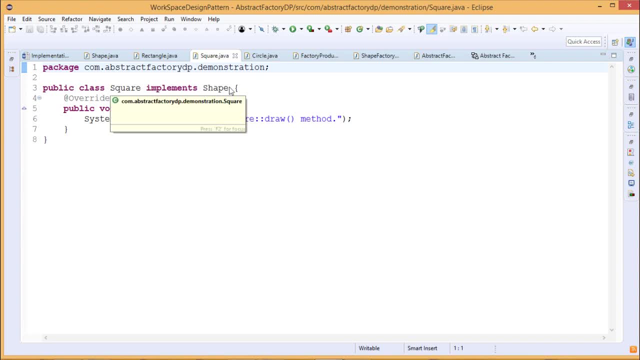 here. so this is a square, is a class which is implementing the shape interfaces javajava and javajavajava. So we have discussed that is, the shape is nothing but one interface and it has got implemented in the class. that is a rectangle dot java, square dot java and circle dot java. So now let us go for the next steps. 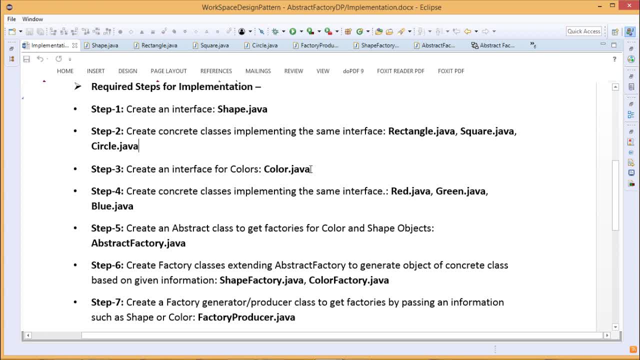 So here we will be defining one interface known as the color dot java, and this color dot java will get implemented in the in three different classes: There is a red dot java, green dot java and blue dot java. So let us go for that implementation. 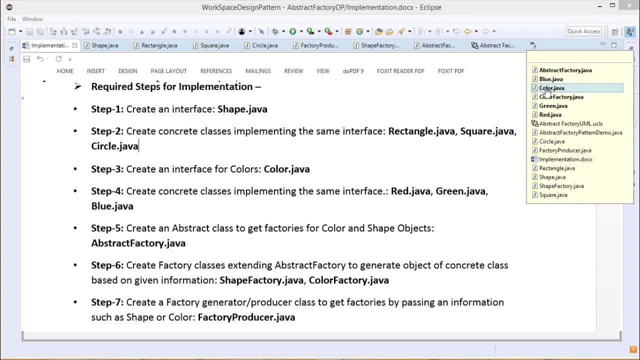 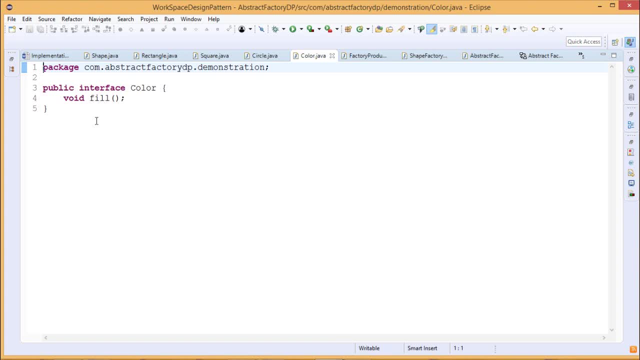 So at first we will be going for this. this is our color. this is a color, is nothing but one interface. It is having only one method, unimplemented method, That is of a fill. So now we shall consider there is a red dot java which is implementing this color interface and the fill method has got its body here. 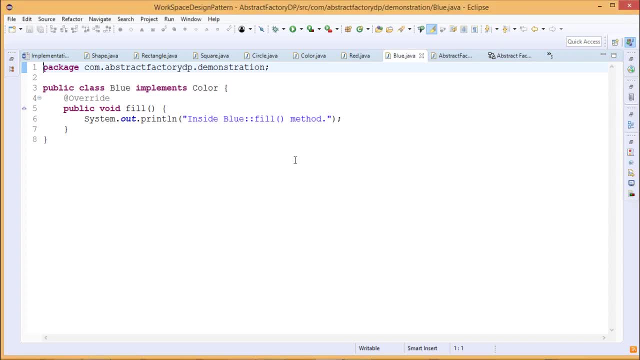 So let us go for another two implementer. So we are having this blue dot java which is implementing this color interface. The fill method has been written accordingly, So we are are going for the next one, that is, the green dot java. so in case of green dot java, it is also 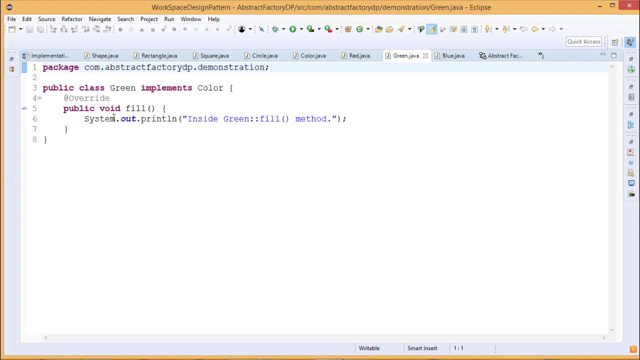 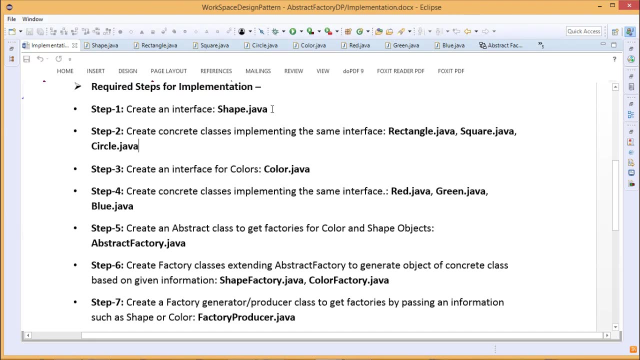 implementing the color interface and the fill method is having this system dot out dot print ln statement here. so up to this part we have discussed, so there is a shape dot java is the interface, rectangle dot java, square dot java and circle dot java are their implementing class and 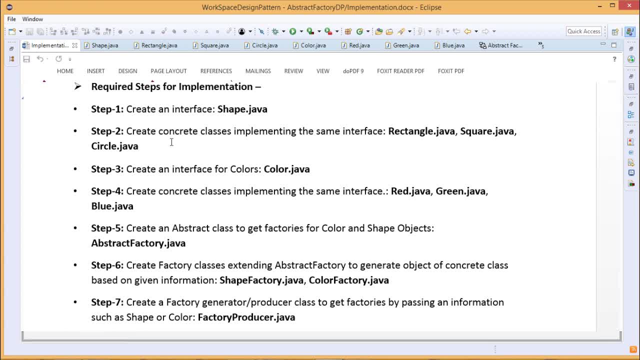 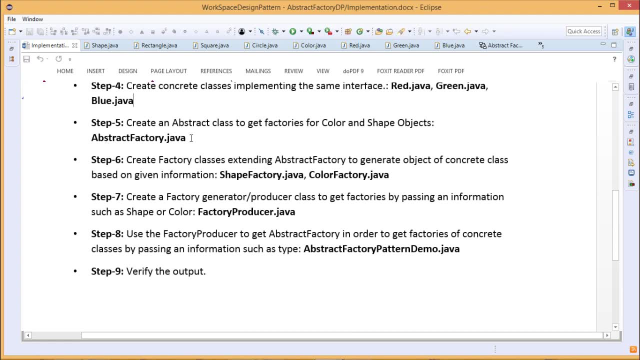 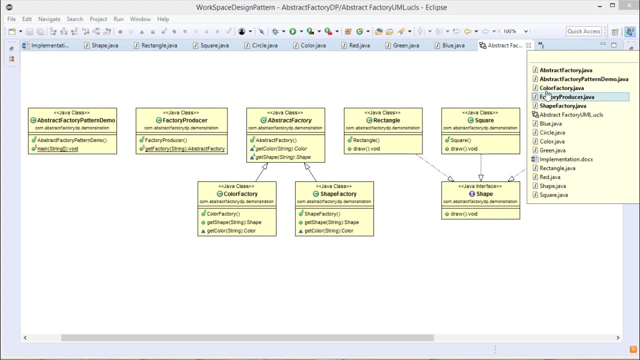 we are having this color dot. java is interface and it is having the implementing class, like your red dot java, green dot java and blue dot java. now we shall go for this abstract factory dot java, okay, so now let us go for abstract factory dot java. so this is my abstract factory dot java here. 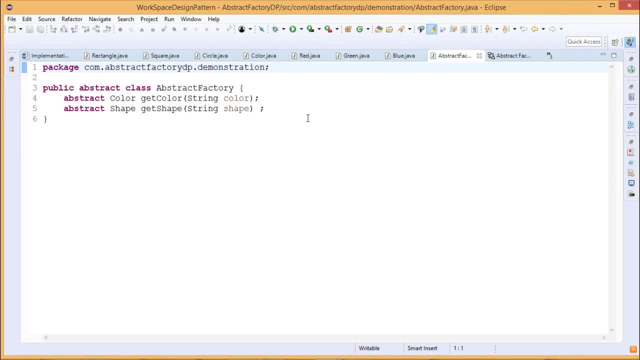 okay, we have got it extra abstract factory dot java, and as it is an abstract class, so its its method will remain unimplemented. the body is not mandatory to be written here. so here you have written two abstract methods. that is the abstract color, gate color, string color. 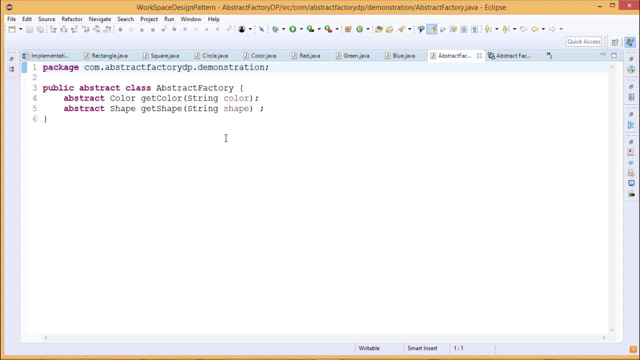 and abstract shape- gate shape, string shape. so we'll be passing some string here as input parameter. so there is a color, a string color in case of gate color, and it is abstract method. so that's why the class is also abstract and as this is the abstract method, so we are not writing the 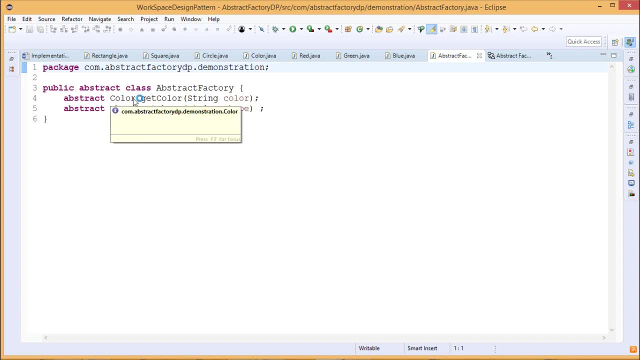 method body here, and it returns color object. so you know that color is nothing but one interface. and similarly, this is another method called the gate shape, which takes a shape string as input parameter and which returns the shape object as output. so this is the respective body for this. 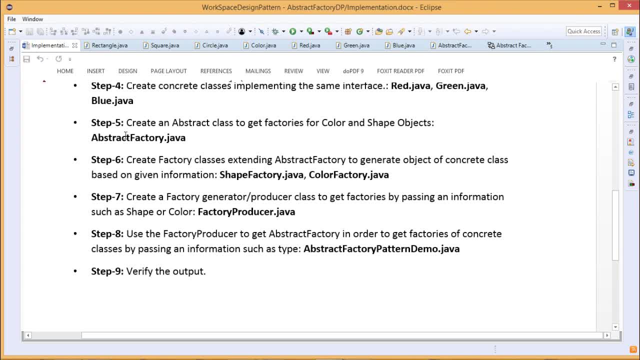 abstract factory. now we shall go for this. so we have completed this abstract factory here. now we will be going for this: shape factory, dot java and color factory, dot java. so create factory classes, extending abstract factory to generate object of concrete class based on given information. so there, 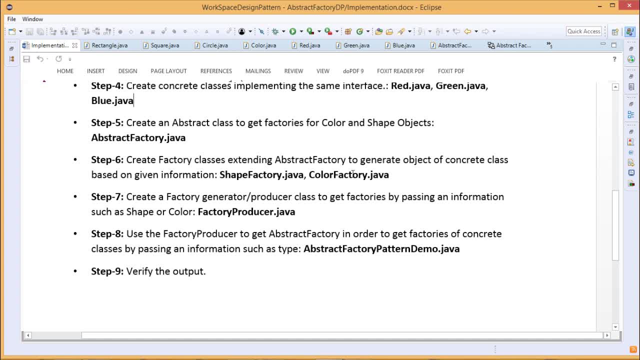 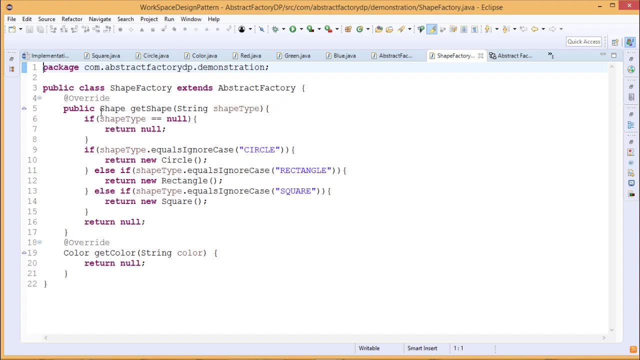 is a shape factory dot java and color factory dot java. they are nothing but the implementing class of this abstract factory, abstract class. so we shall go for the shape factory dot java. so there is our shape factory dot java, which extends abstract factory, abstract class. so here, this is a method we are having. there is the gate shape, so depending upon the string which will be, 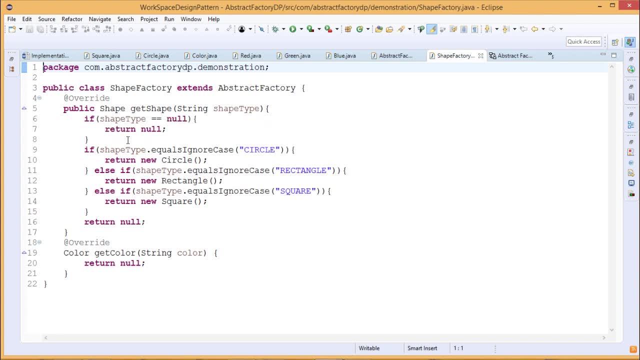 passed as the input parameter, the required shape object will be returned. if the input parameter is null, it returns null. so shape type: dot equals ignore case. so if the, if the string is circle, the, then it returns the circle class object. if the input parameter is string is rectangle, it returns. 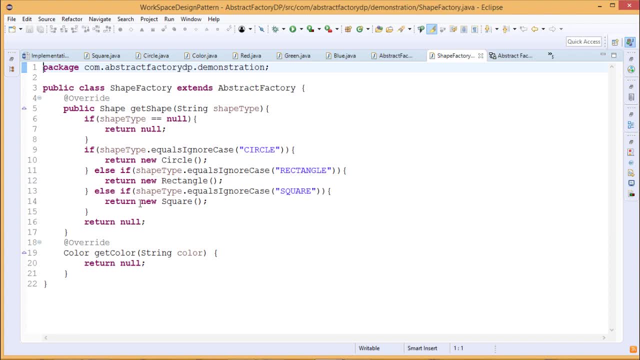 rectangle class object. if the input string is square, it returns the square class object, otherwise returns null. so this is a respective method body for the gate color, which returns null. so there is no such business logic. we have written for the gate color. so that is the class, that is the shape. 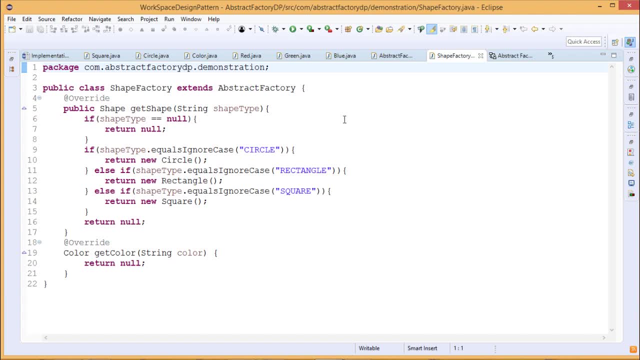 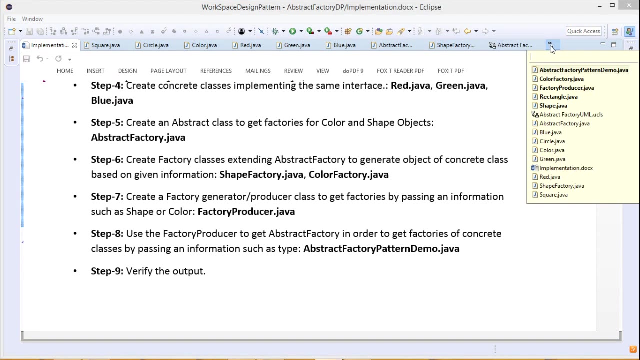 factory which extends the abstract class, abstract factory. so now we shall go for the other shape one. so there is a shape factory here. so i shall go for this, the shape factory, and then we will be going for the color factory. yes, so there is a color factory. 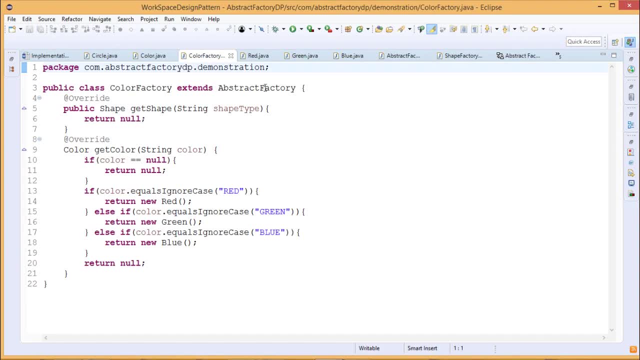 here. so this is a color factory which extends the abstract class. that is the abstract factory. and here, in case of gate shape, we have just written null. no business logic. we have written here no. if then else, but in case of color, gate color, this method, that is a string color, will 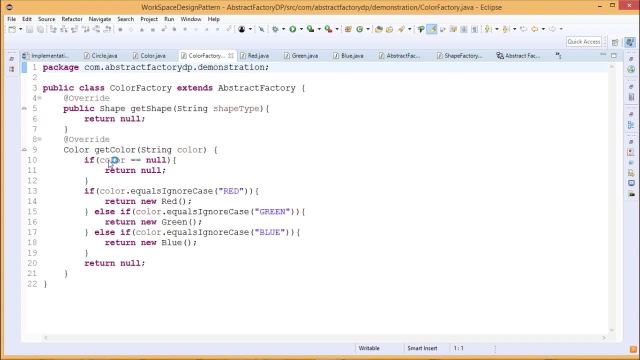 be passed as input parameter if the color is equal to null. if the input parameter is null, it returns null. if the input parameter color, which is of the type string dot, equals, ignore case red, it returns the rate class object as output argument. otherwise, in case of green string, it returns the green. 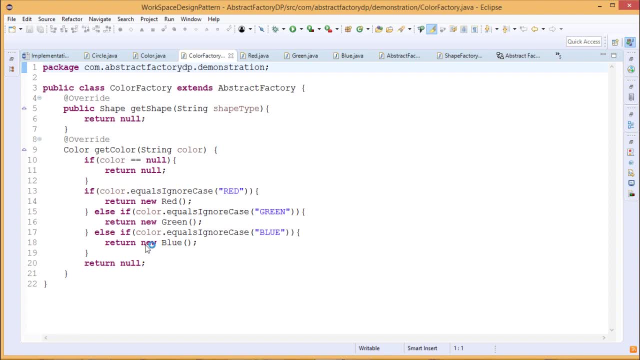 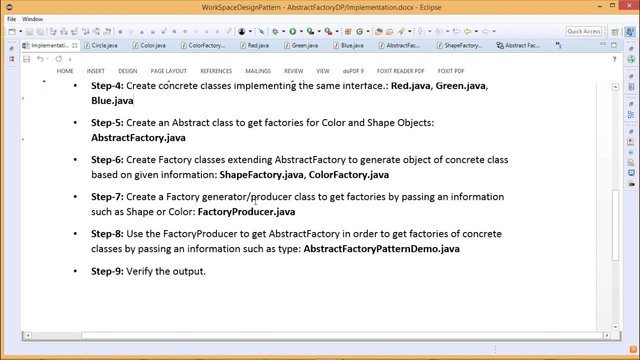 class object as output and if the string is blue, it returns the blue class object as output argument. otherwise it returns null. so we have, we have gone through up to step number six. now we are coming to the step number six. we are moving to step number un quaków. step number five. 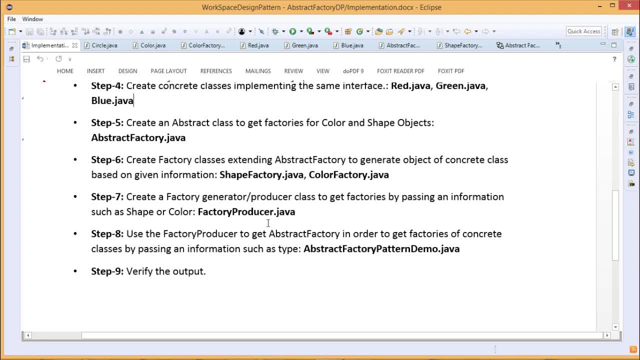 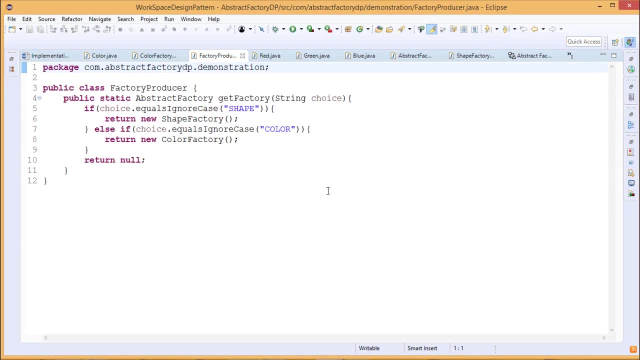 Number seven. so create a factory generated or producer class to get factories by passing an information, passing an information such as the shape or color. So here the name of the class will be factory producerjava. So now let us go for this: factory producerjava. 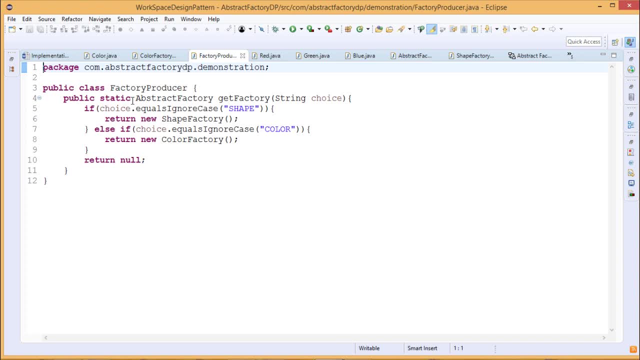 So public class factory producer. So it is having one method. There is a public static abstract factory- The name of the method is get factory- which takes the string as choice, as input parameter. So if the choice dot equals ignore case shape, then it returns the shape factory class object as output. Otherwise it returns the color factory class object as output. Otherwise it returns null. 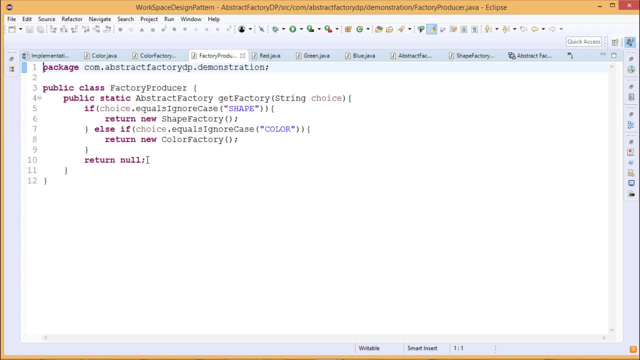 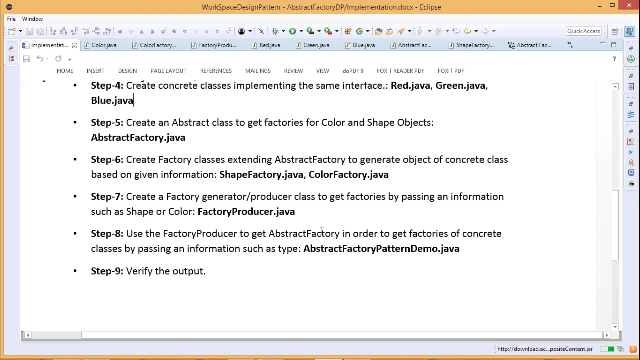 So actually it is returning the shape factory, This shape factory class object as output argument If the input parameter is shape. otherwise, if the input parameter is color, it returns this return: new color factory. There is a color factory class object as output. Otherwise it returns null. The name of the method is get factory. defined under the class There is a factory producer. So now let us come to the step number eight. So that is the last but one step: Use the factory producer to get the abstract factory in order to get factories. 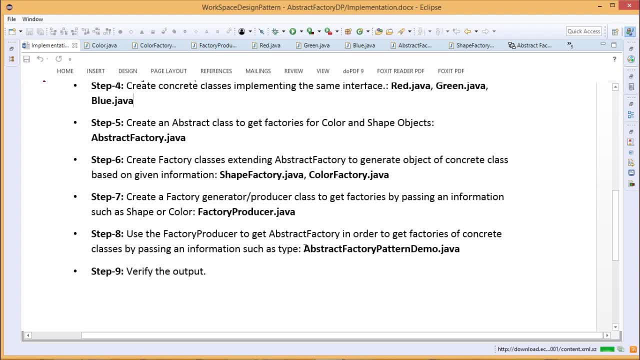 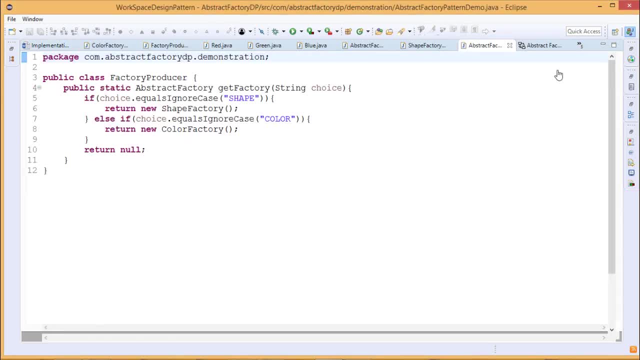 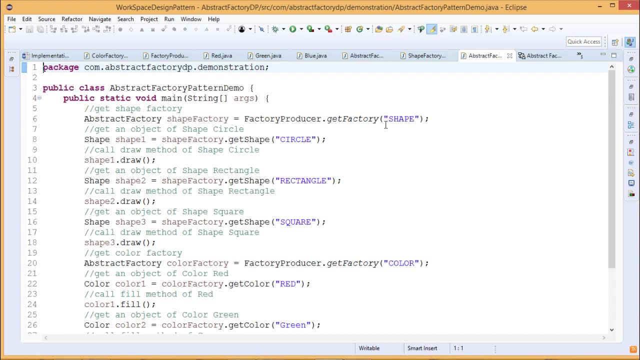 Of concrete classes by passing an information such as type: abstract factory pattern, demo dot java. So here we are going for the final class here. So now, here you see, we are having this abstract factory shape. factory is equal to factory producer dot get factory shape. So as we have passed the string shape, So it is returning the respective object, So you can also find it here. 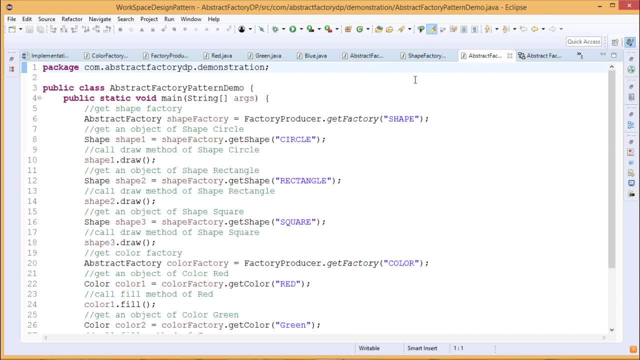 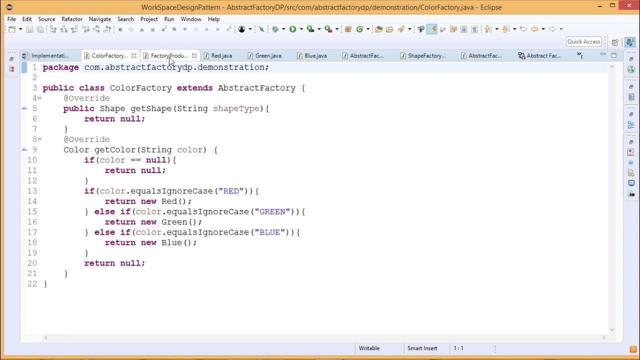 So whenever you are passing this, this, uh, i'm just going for this factory producer. okay, so let me go for this implementation: color factory. you know, this is a color factory. there is a abstract factory extends. this is a factory producer. depending upon the input string shape. 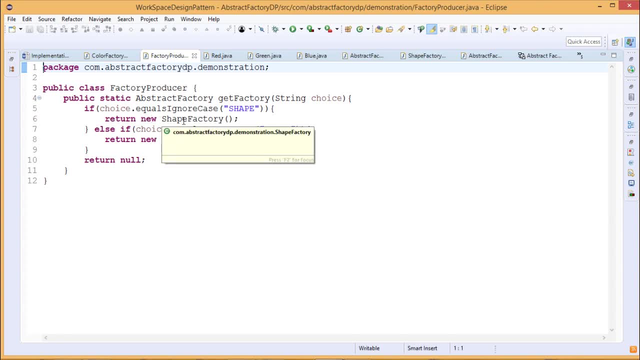 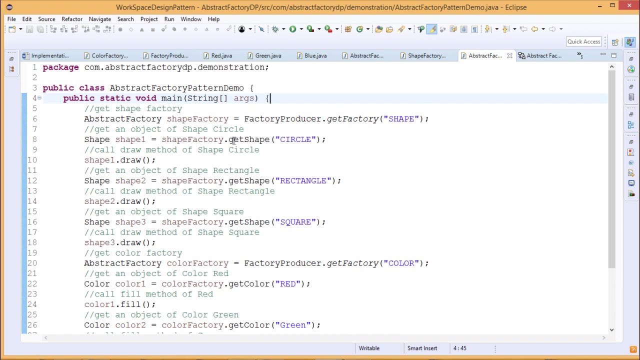 it returns the new shape factory there is: the shape factory class object will be returned if the input parameter is colored, returns the color factory object as the as the output argument. okay, so that's why, as we have passed this shape, so it returns the respective class object as. 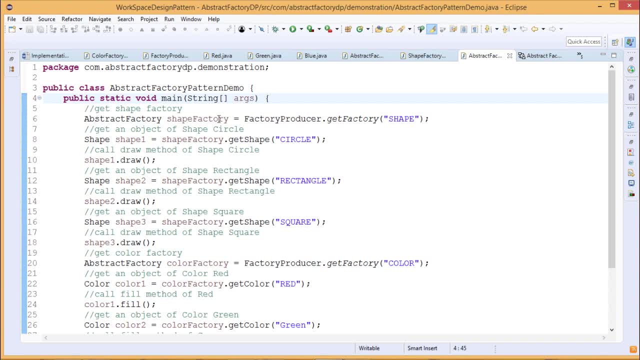 as the output argument and that has been kept in the shape factory. so now shape factory dot get shape. i pass this input string as circle, so whenever we are calling this shape one dot draw, we are getting the required output like this. so insert inside circle: colon, colon. 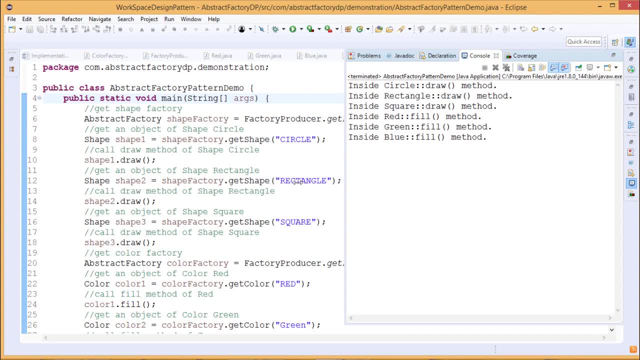 draw method is getting executed whenever we have passed this input string that is a rectangle, as input argument, so whenever. so that has been kept in shape shape two and then shape two dot draw. it is just printing this inside rectangle: colon, colon draw method. that means the respective 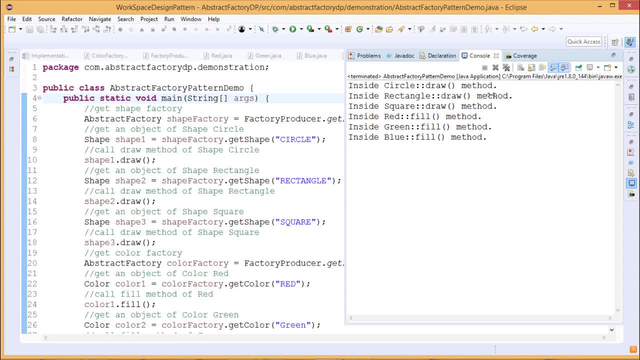 rectangle class object. within that, the draw method which was defined the, that that very method is getting executed. so whenever we are passing this rectangle as the string, as input argument to this get shape method, which is defined under the shape factory, so get shape method. so now what is what is happening? it is returning the rectangle class object as output. 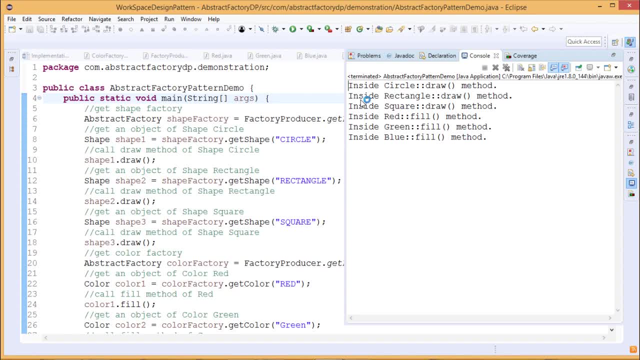 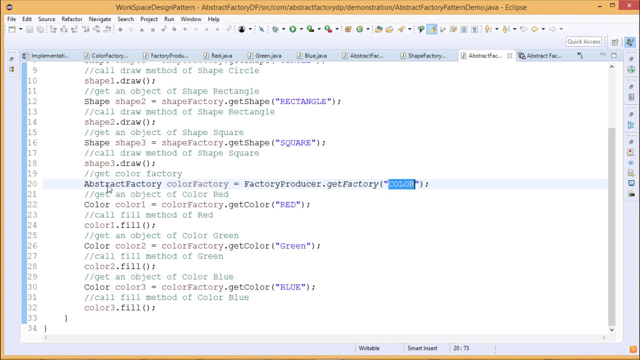 so whenever you are writing this shape two dot draw, it is executing the, the draw method which was defined under the rectangle, under the rectangle class. so similarly for this red. so here we are passing this color, so it is returning the respective class object as output, which has been 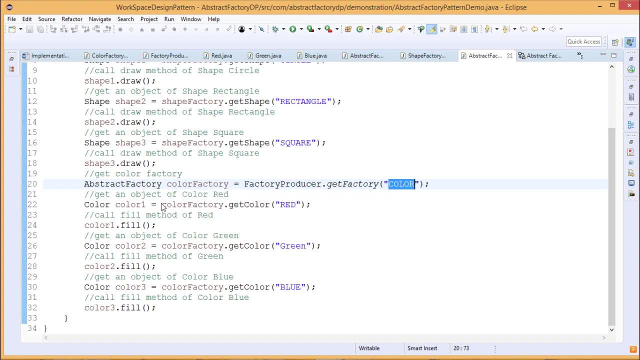 abstract factory, that is, a color factory, here and whenever, whenever you are calling this, get color, passing this red as input argument, and then, whenever we are calling this fill method, we are getting this output like this: so that is the inside red colon. colon fill method is getting. 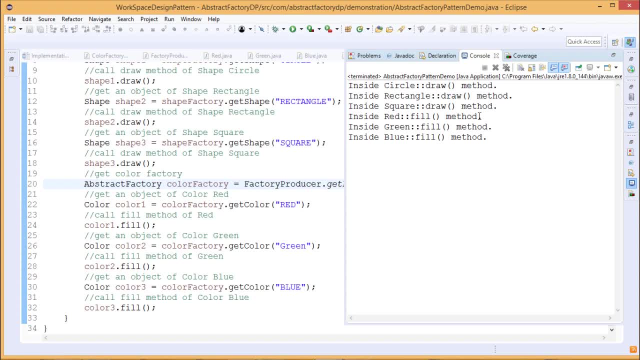 executed. so that means it is. it is that very method, that is a fill method, which is implemented in the red class. and we know that red class implemented the color interface which have shown in the uh in our coding. so, similarly, when you are passing this green as the string, as input parameter, so it is. 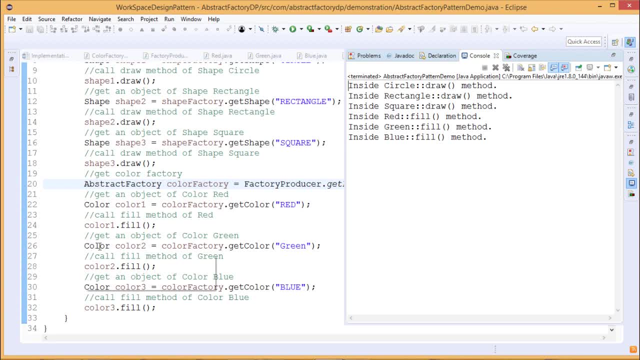 returning the color object. and you know this color is nothing but one interface. but as this green is the string which has been passed, so the respective green class object will be created and that will be dumped on this color two. so whenever color two dot fill is getting executed, we are getting this. 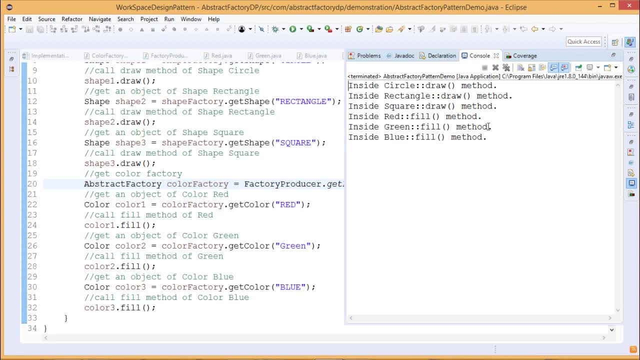 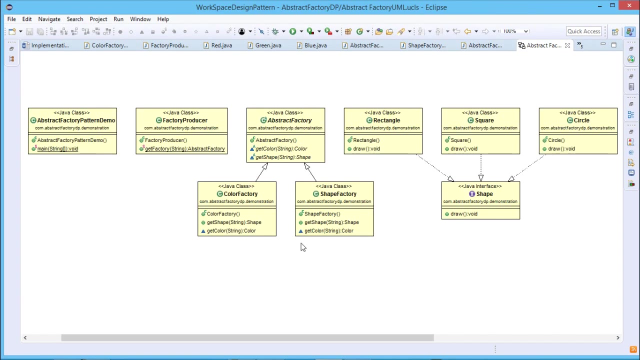 string that is, the inside green colon colon fill method is getting executed. similarly, we are getting the output when the input parameter is blue string. so in this way we have we are given the idea that how this abstract factory design pattern can get implemented. so these are respective. 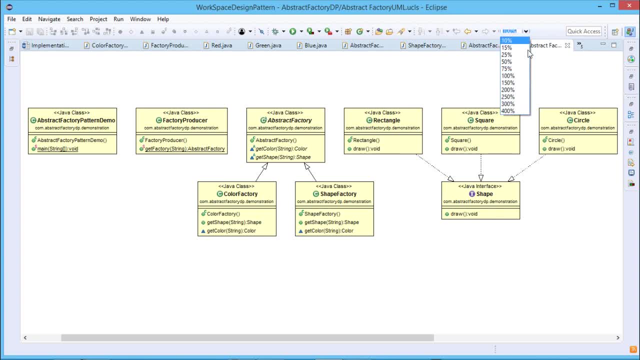 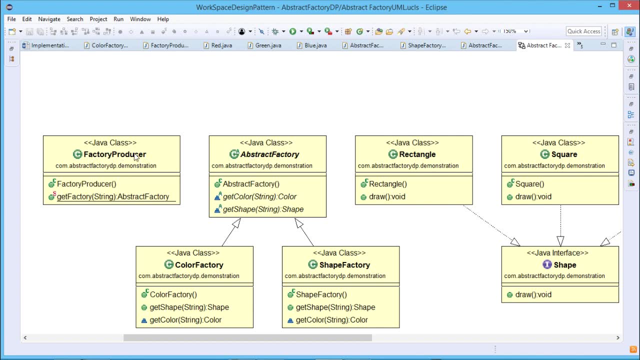 use case diagram. you know this is a class diagram, rather so if you go for the little bit zooming here. so there is a factory producer, so we are having this. there is the java class factory producer, we are having this abstract factory and there's a color factory and shape factory, so we're having